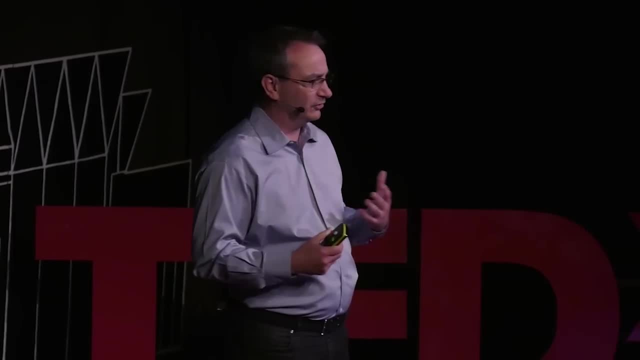 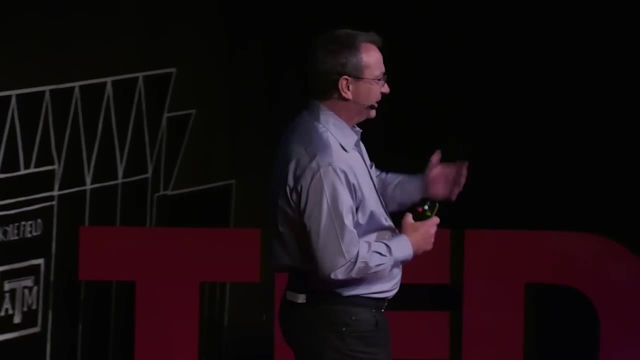 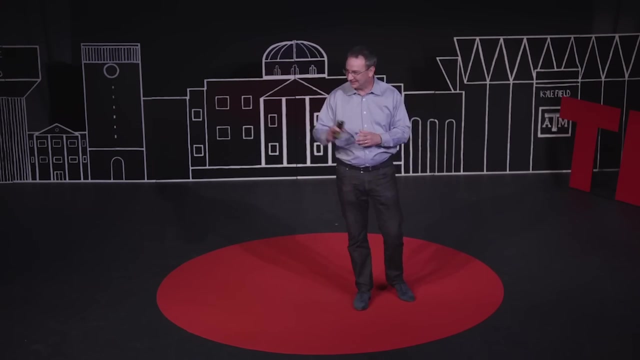 things have really changed, So why is education not really moved forward in this rhyme? Anybody know what this is? Periodic table of elements. How many elements in there? 110, 140, 180, so somewhere between 100 and 130 maybe. 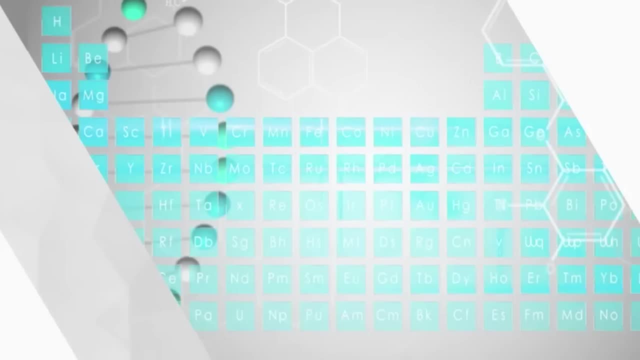 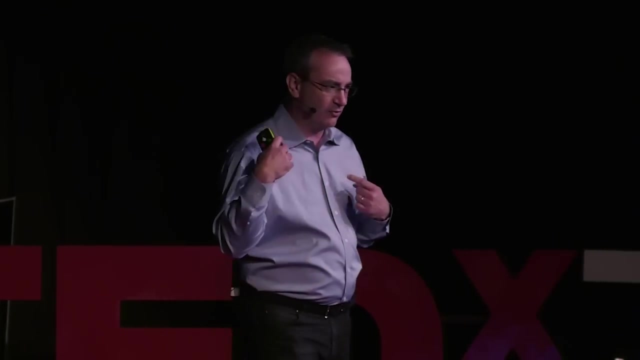 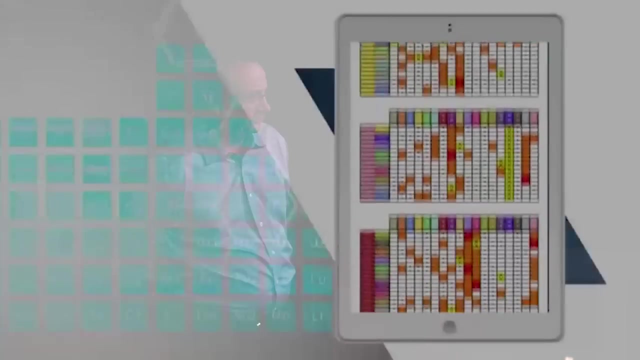 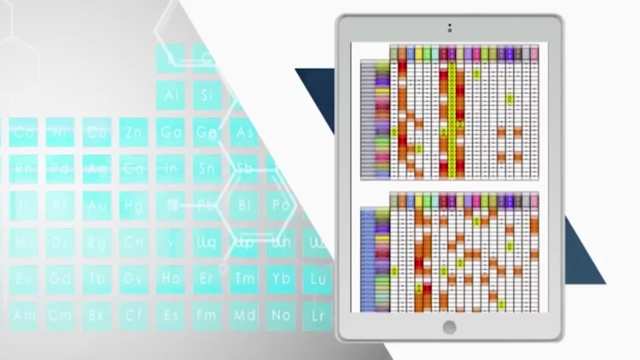 We're all supposed to learn this. What does it actually say? What do these boxes actually mean? It's a chart and we're supposed to know what it is. Well, let me show you another chart in comparison. It keeps on going and going and going. It's still going. It's so big it doesn't. 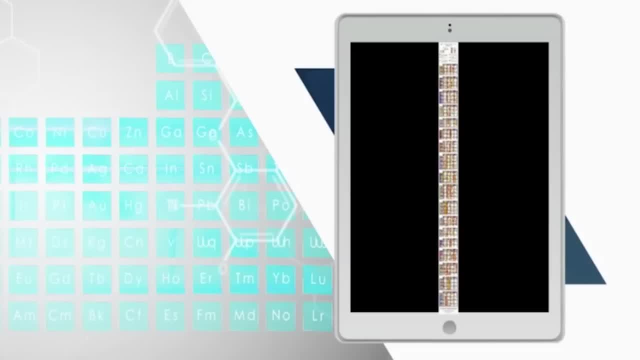 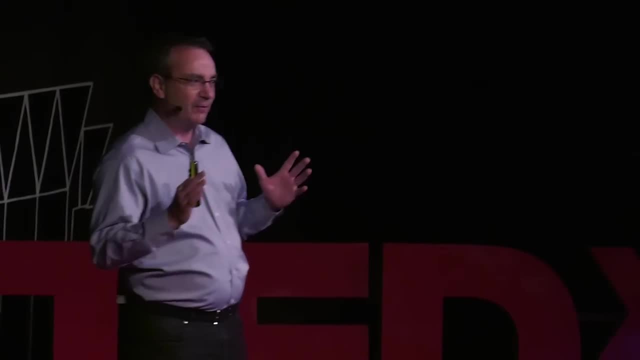 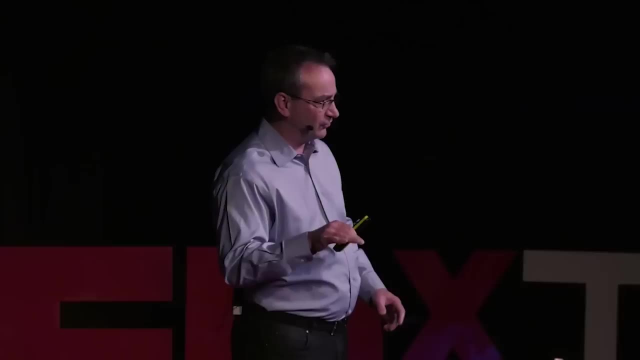 even fit on the screen. What if I told you you have to learn this chart and know by heart? Oh, great, right, teacher, wonderful. But what if I told you ten-year-olds know this chart by heart? What if I told you? 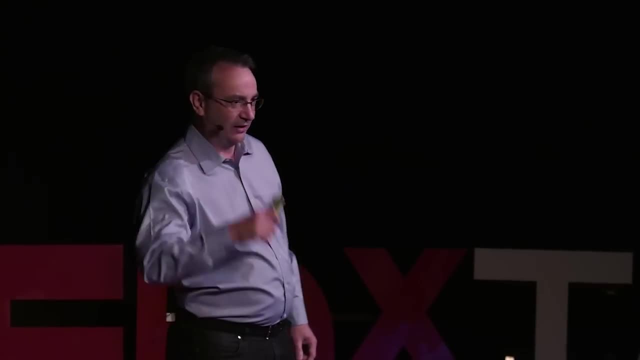 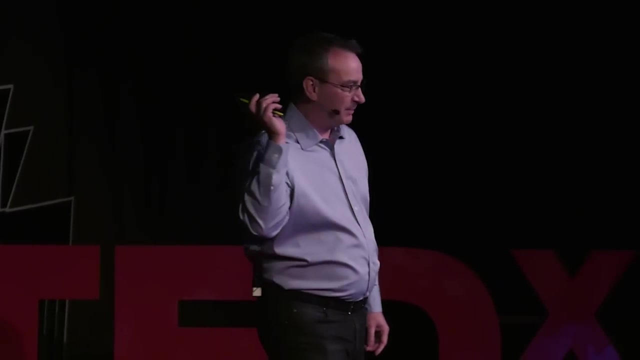 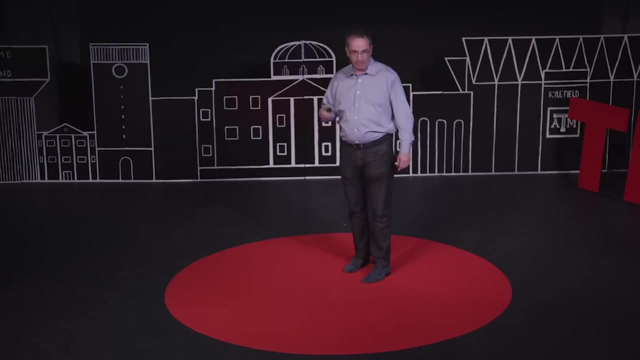 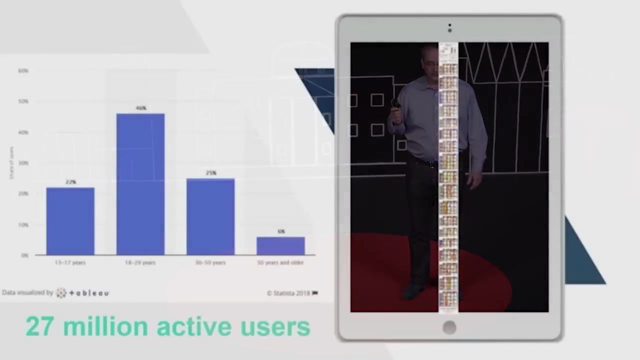 ten years later, they still know this chart by heart Because I didn't have to learn a chart. That's a dual type. abilities from Pokemon, Again hugely popular. and there's the data behind it: Even today, over 27 million active users. 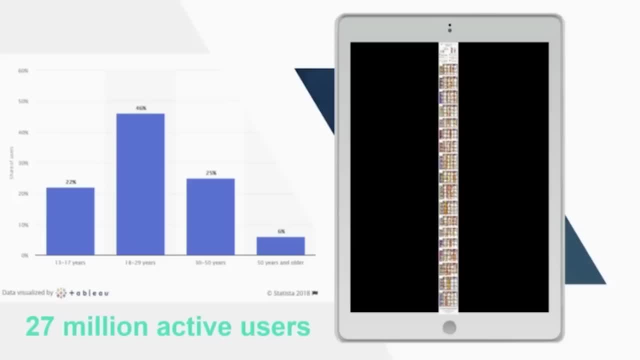 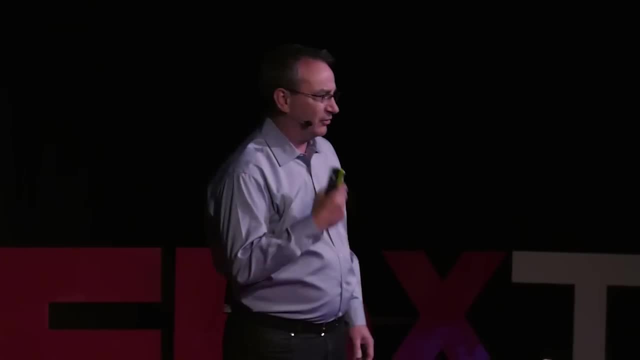 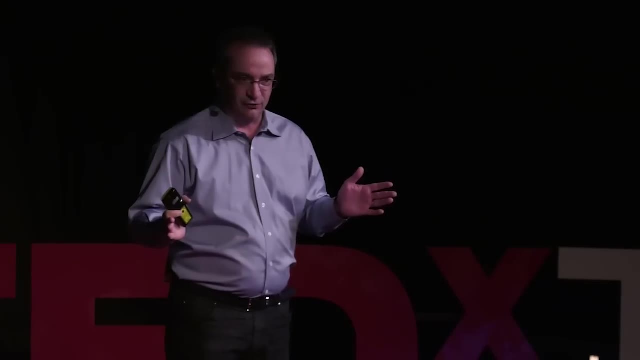 Pokemon, really That chart. periodic table of elements: 118 elements we can't remember. yet ten years later, they still know this by heart. That's the power of games. Now I hear you may say games don't really belong in the classroom. Well, that's. 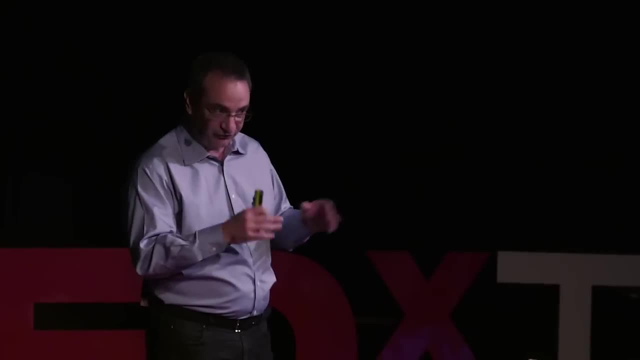 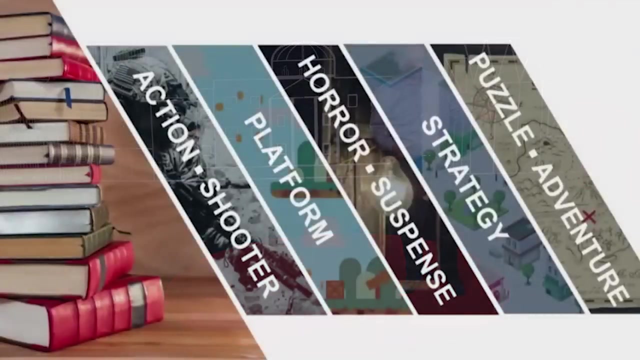 like saying books don't belong in the classroom. I don't prescribe to that, because games are a medium, just like books. You have all types of books. You have recipe books, You have textbooks, You have reference books, You have comic books, All different types of books. 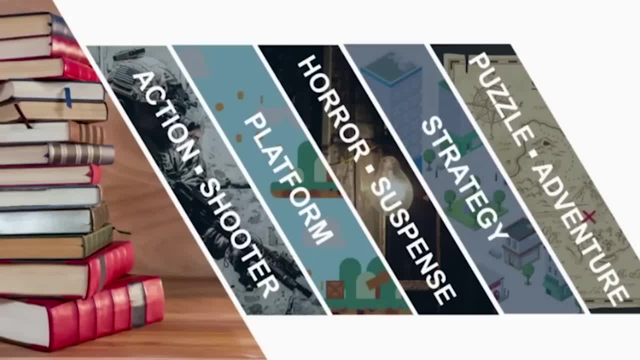 All different types of books And we have the same with games. We have all different types of games. We have puzzle games, We have adventure games, We have first person shooter games And we have games for learning. Let me show you some examples of games. Here's. 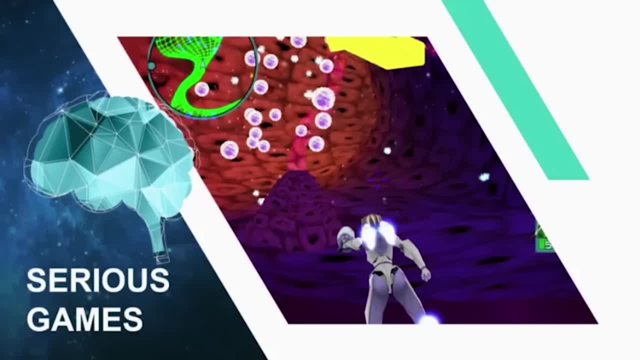 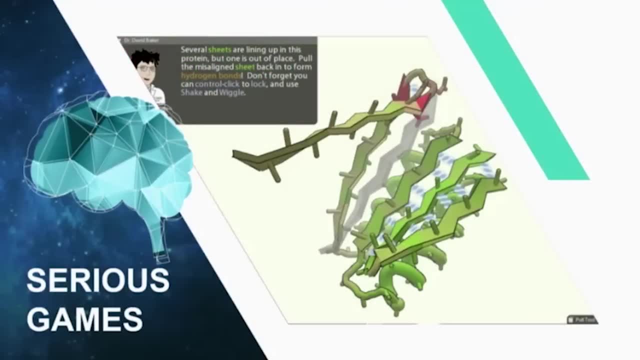 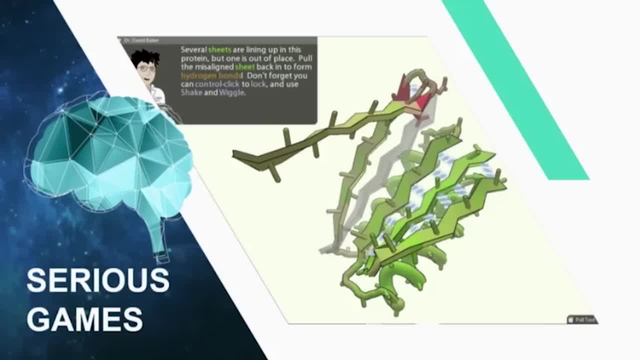 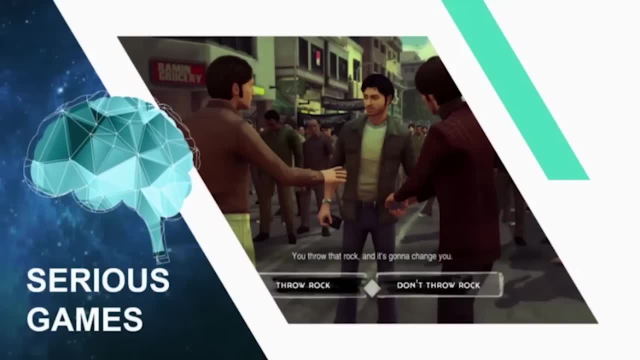 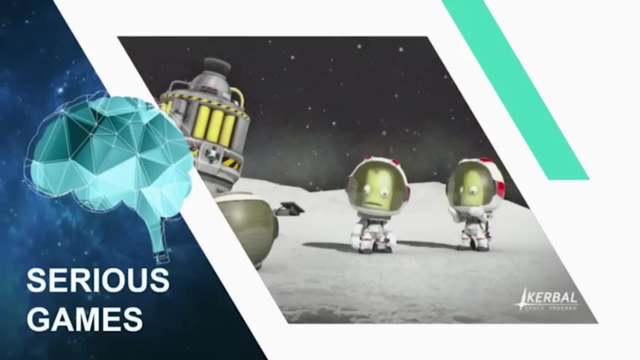 A game where players help scientists discover new proteins. A game for science, 1979.. You take on the role of a journalist in Tehran and see the Iranian Revolution from a very different perspective. Call it the historic or documentary game, And some of you may know. 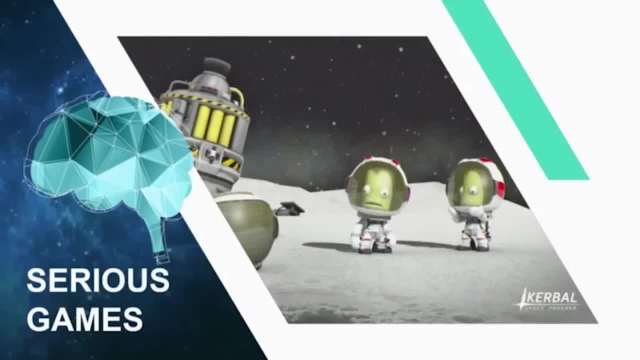 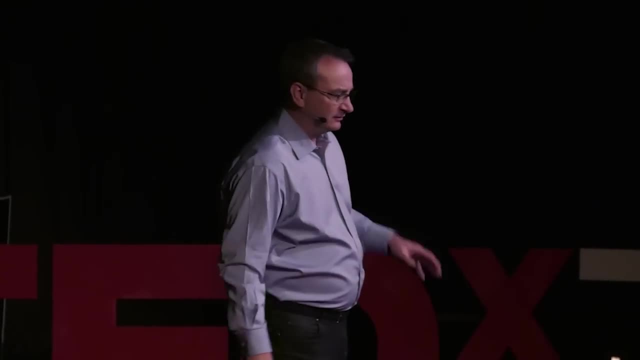 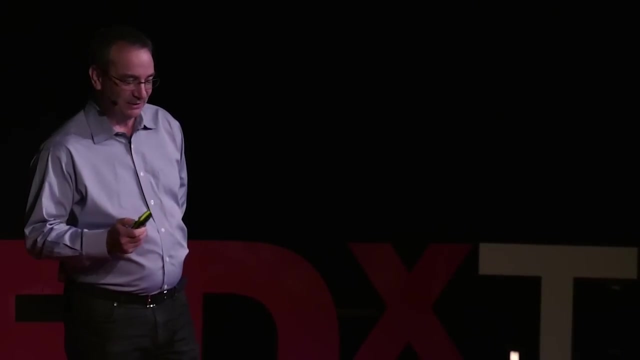 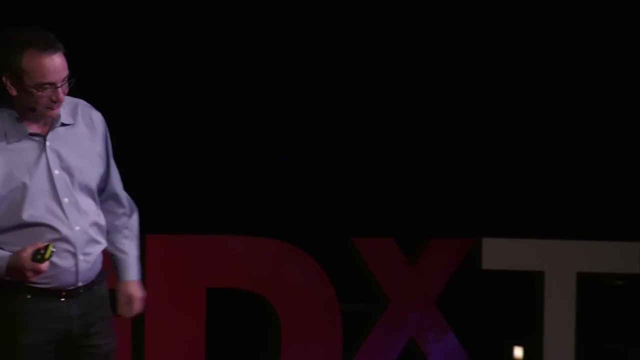 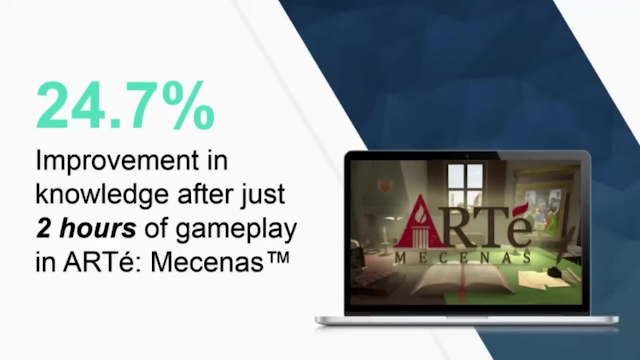 this game- Kerber space program, So Bereich children- and it helps. Let me show you an example that was created right here at Texas A&M. Okay, maybe not Okay, the video didn't work, Okay, but we created the first ever art history game right here at Texas A&M in the Life Lab. 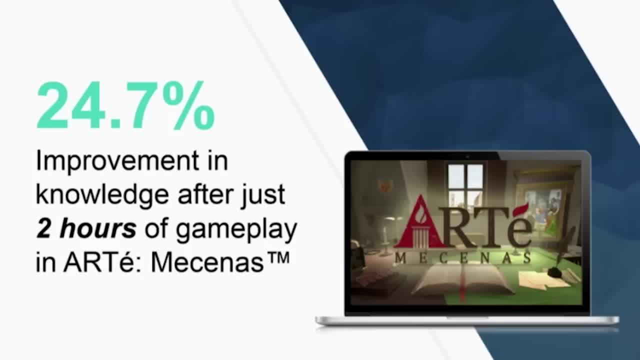 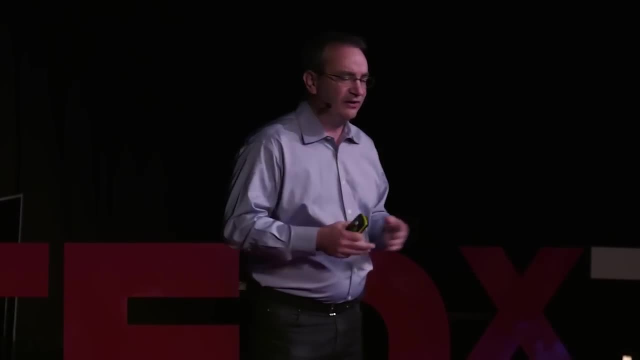 with our students, with faculty and with the help of Triseum. That game has shown research that we conducted 24.7% of student improvement after just two hours of gameplay. Why did we create the game? Well, here we have art history survey classes. These are large lecture classes. 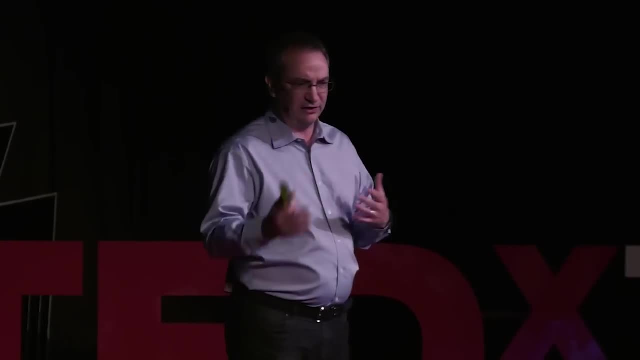 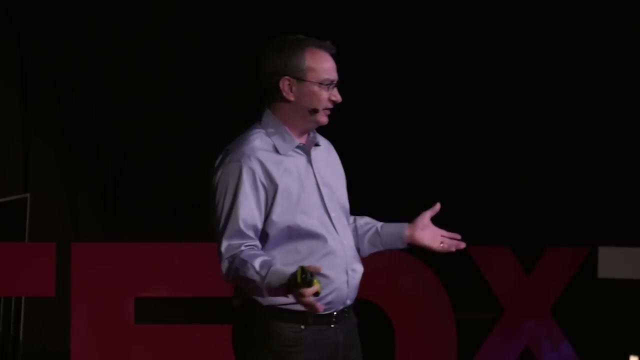 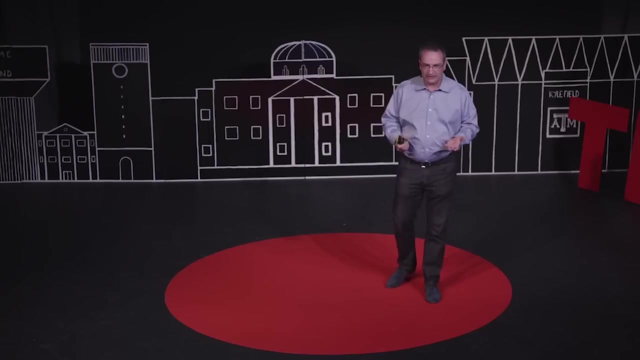 where students get introduced to art. These are engineering students, business students, architecture students. The only time they ever hear about art is two semesters, five thousand years of art, human art history. There's only so much they can get out of it. It's like trying to see Europe in a speed train in a week. 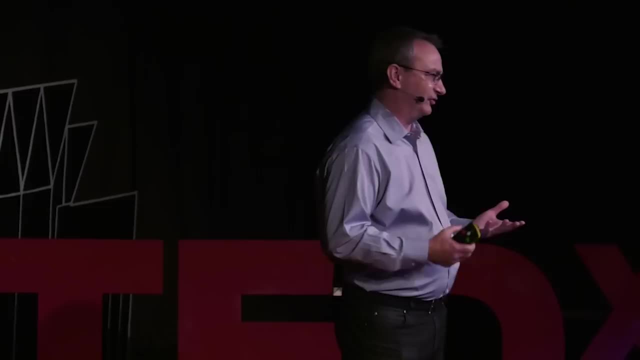 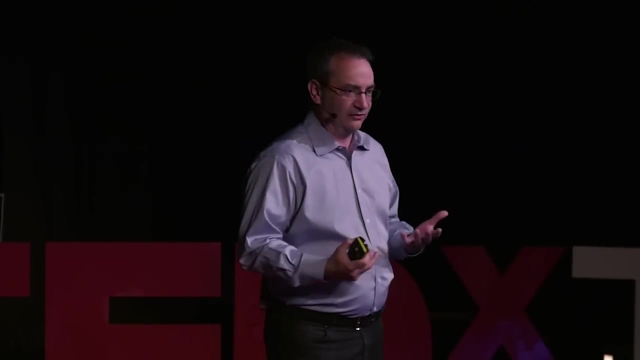 How much are you gonna remember, How much you're really gonna understand about Europe? So the teacher, the professor that teaches art history, thought: well, maybe there's a better way to engage with our students, to bring deeper context to the students through games. 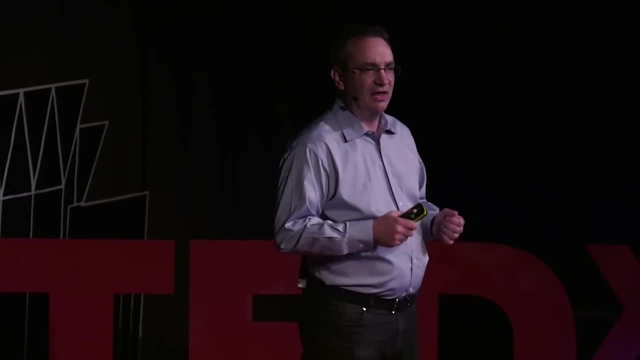 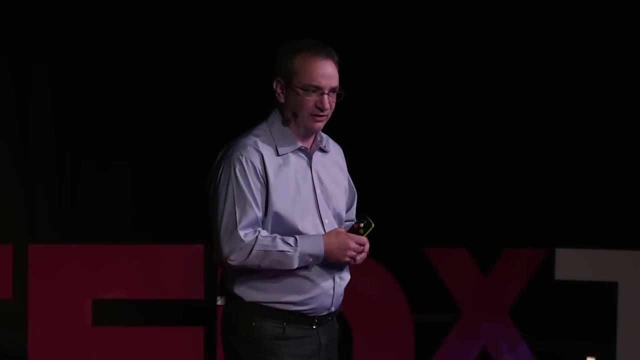 Knowing that 97% of students play games every week four hours or more, That's boys and girls. Now, they don't necessarily consider themselves gamers. Playing Candy Crush? Oh no, I'm not a gamer. but I play Candy Crush. Solitaire, Yes, sure, but I'm not a gamer. 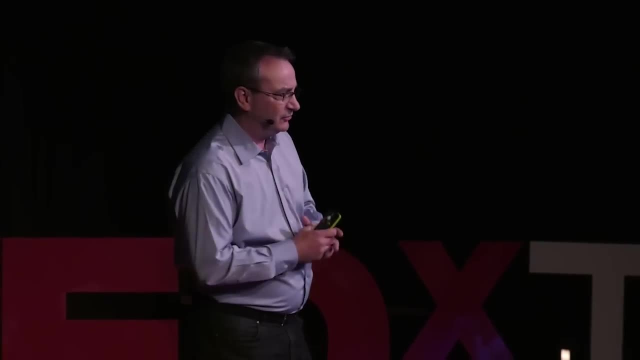 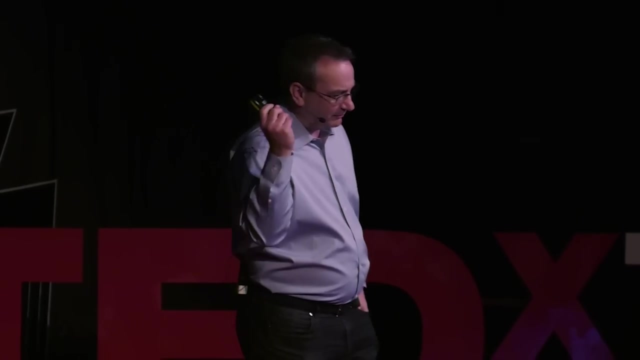 You know, there's all kinds of games- board games, card games, video games- and we can utilize that power very effectively. Let me ask you different. Oh, here's some responses, because this game has been used in classes and universities. 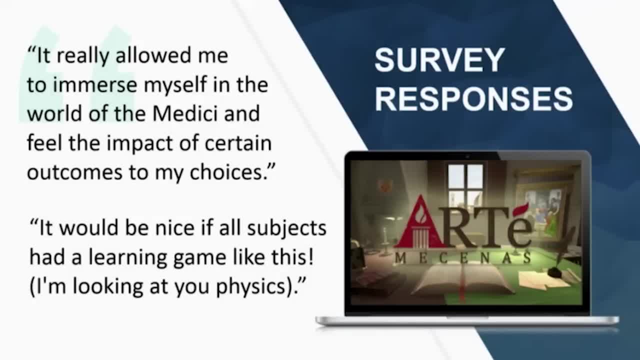 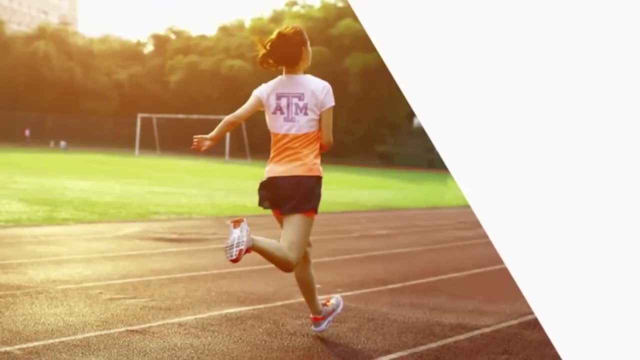 all around the country and now all around the world. In Poland, actually, teachers are using this game to teach English to her students Right here, coming from Texas A&M. What about other subjects? Can we do that? A hundred meter race? if you run 90 meters, what do you get? 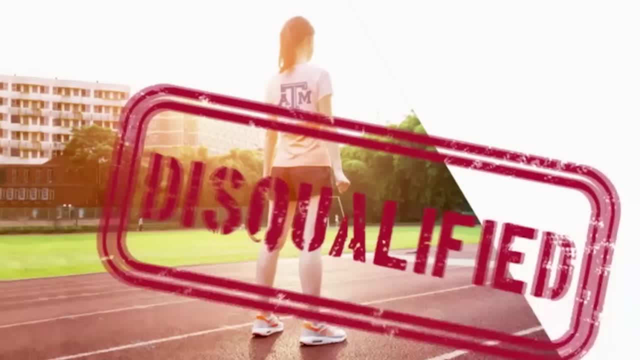 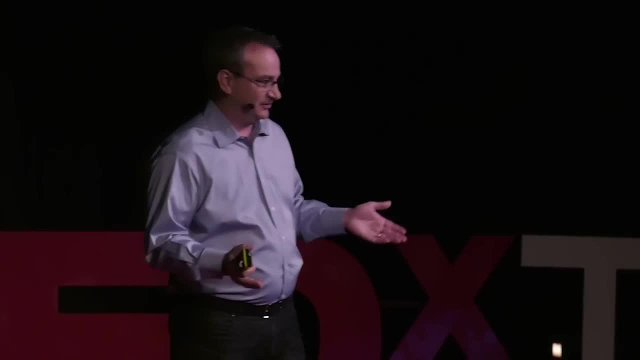 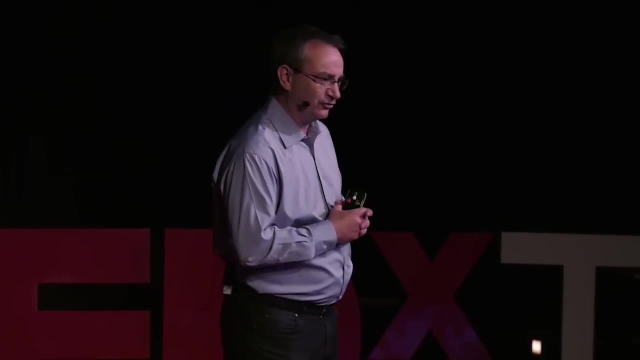 Nothing right. Disqualified. You don't even get last place because you didn't finish 90 meters in a hundred meter race. Well, that's 90%. What do you get in a classroom if you get 90%? 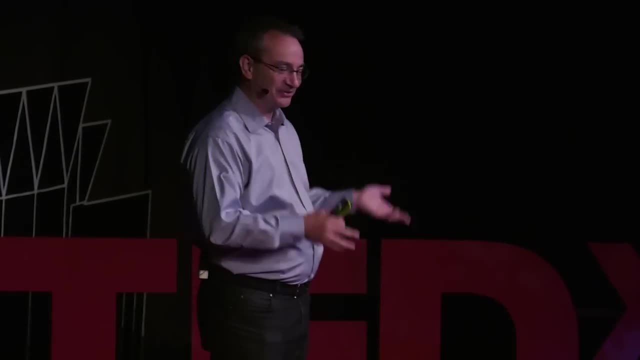 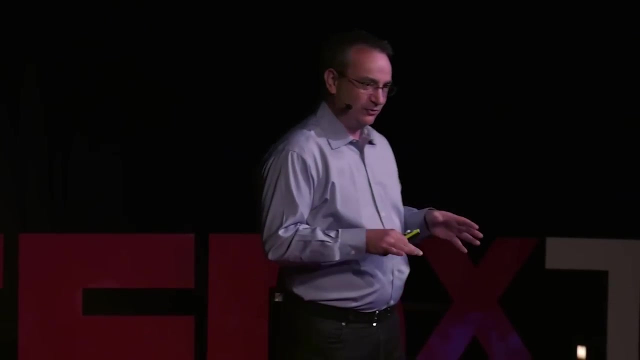 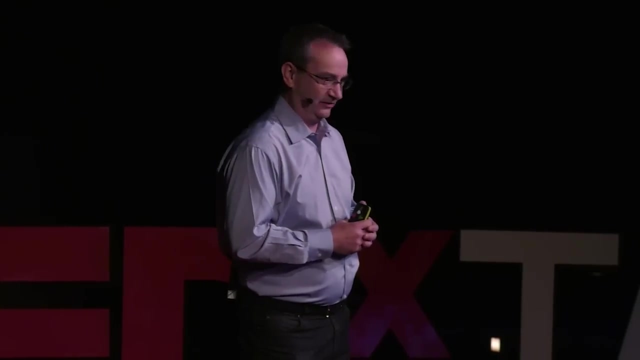 An A. that's right. 90% will get you an A. Yet you actually only got 90%. What if I told you that airplane you're about to get onto it's an A pilot. he's mastered the airplane 90%. 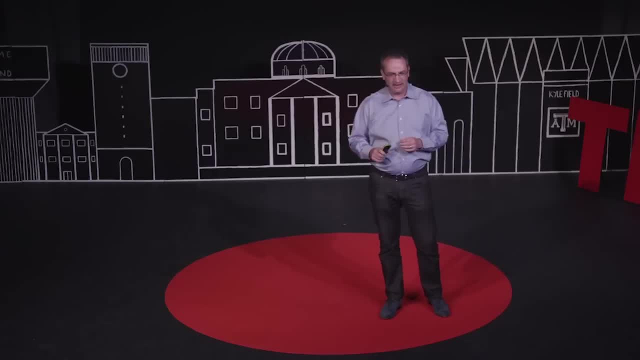 Oh and, by the way, don't worry, the plane is in really great condition. It's 90% working. How are you going to feel about that? I'm not going to feel that good about it. Thankfully, pilots are not educated that way. 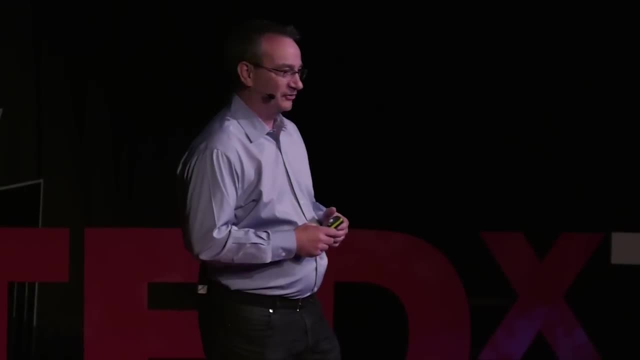 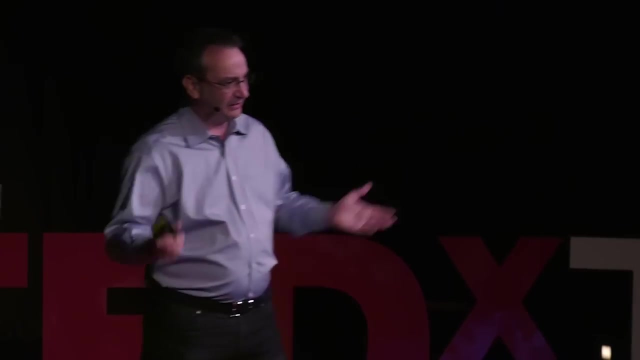 They're educated based really on mastery of the subject, Not 90%. We don't do anything in the real world 90%. Everything is 100%, But in education 90% And that's the A students, Imagine the B students, C students. 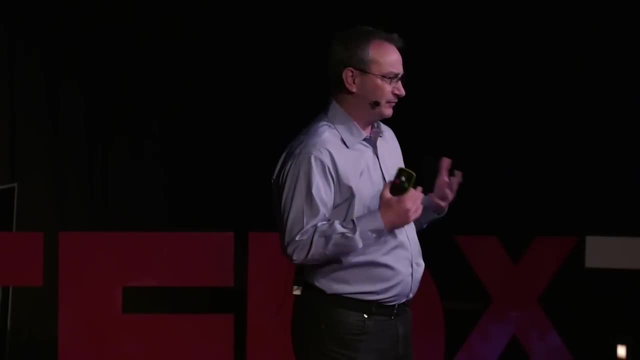 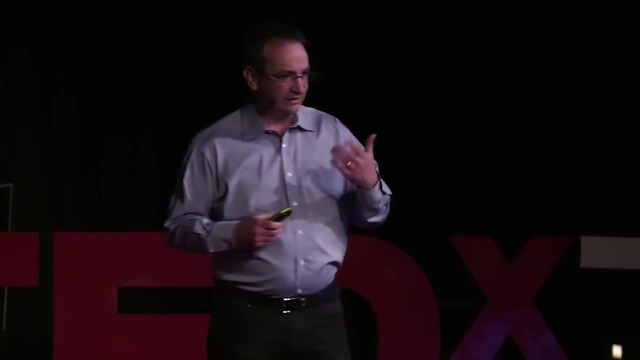 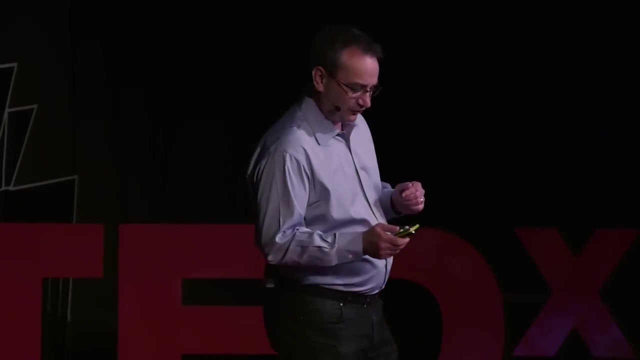 And compounding works in education the same way as it does in finance. Over the years, the knowledge we leave on the table stacks up year over year over year. I'm about to show you another example of a game that was created right here and used. 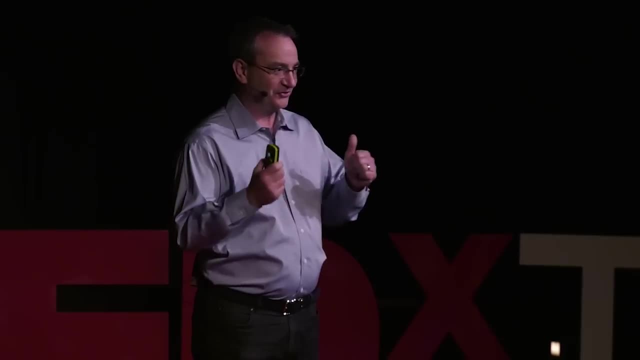 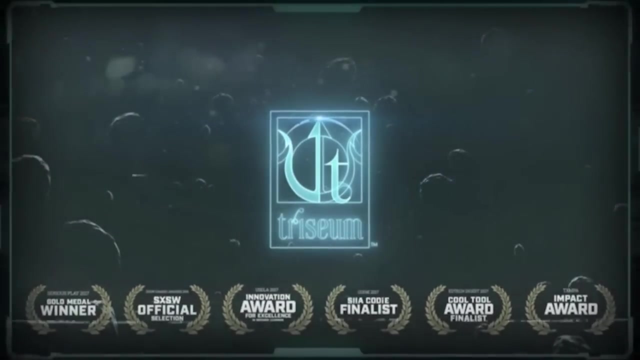 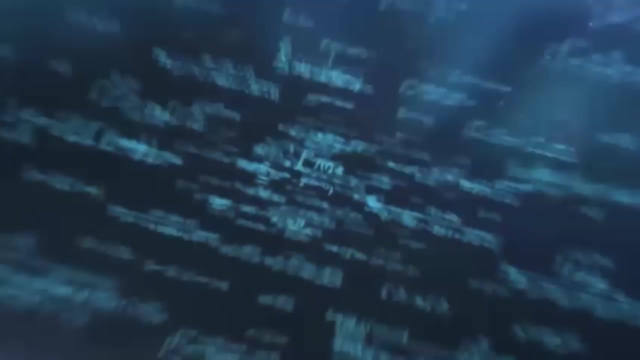 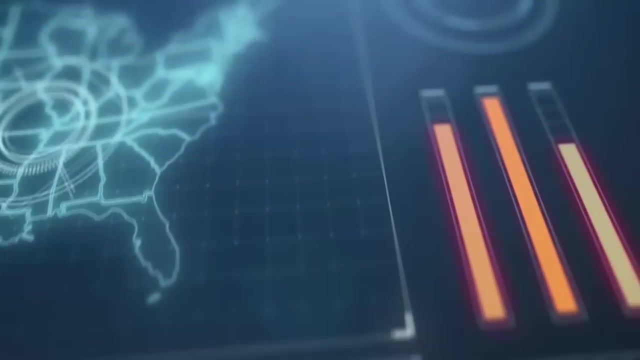 See if this works. Yes, From engineering to medicine to 3D graphics, calculus is foundational for all STEM careers. However, calculus courses today have among the highest failure rates of any course on any campus, And there is a growing body of evidence that explicitly ties calculus. 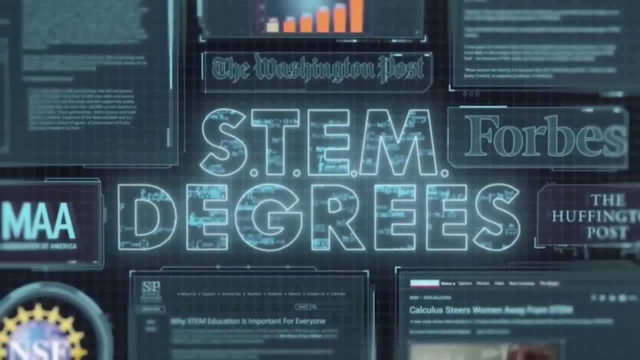 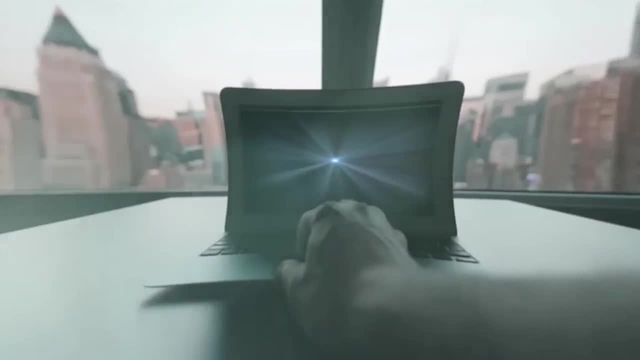 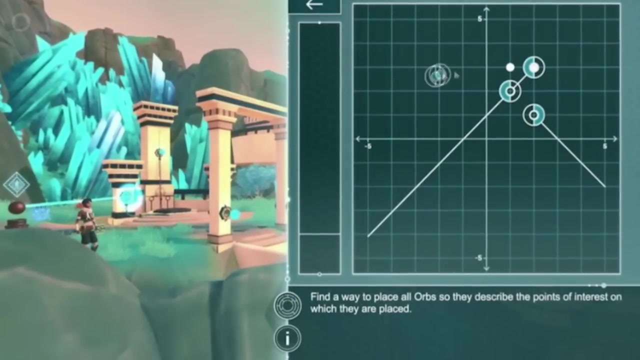 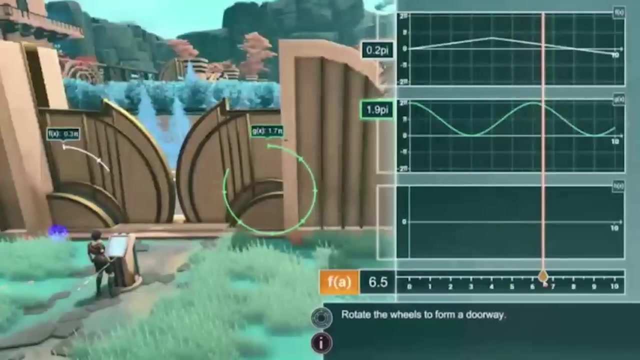 to attrition in STEM degrees At Triceum, our team collaborates with educators to address these complex educational issues and transform how students learn. Welcome to Variant Limits, The first in a new series of immersive educational experiences for calculus students. Variant Limits brings calculus to life by transforming abstract ideas into creative and visually engaging challenges. 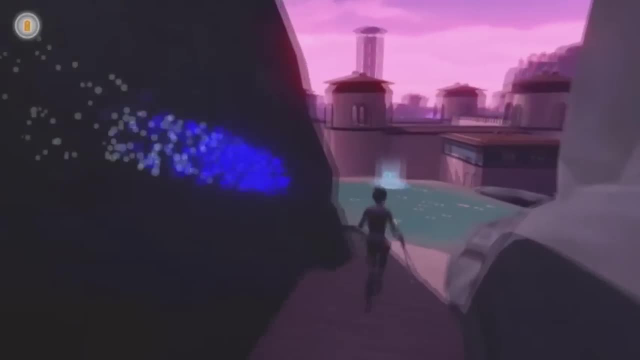 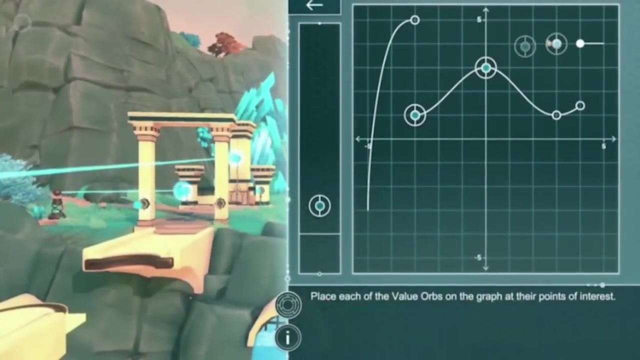 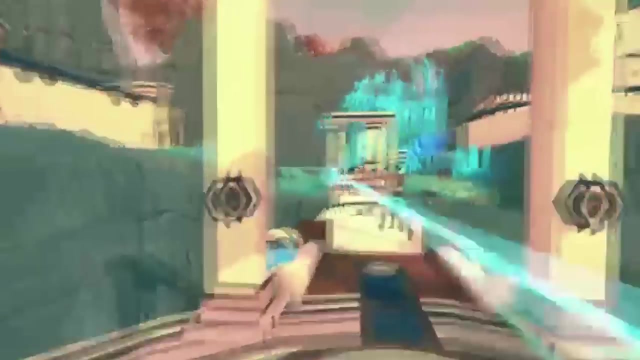 As an explorer on a planet governed by calculus principles. students will discover a vibrant 3D world Throughout the world. students will overcome obstacles by applying skills and concepts learned in class. Students will gain a new perspective on difficult topics such as limit laws, continuity and the intermediate value theorem. 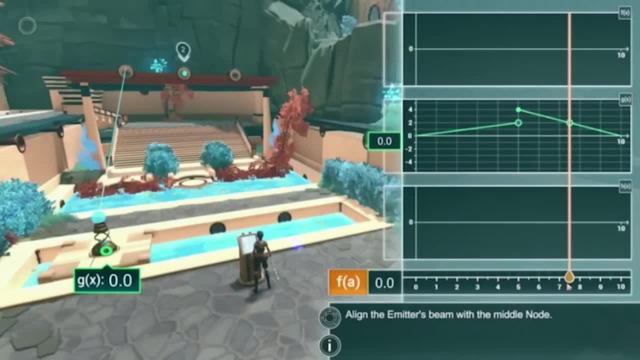 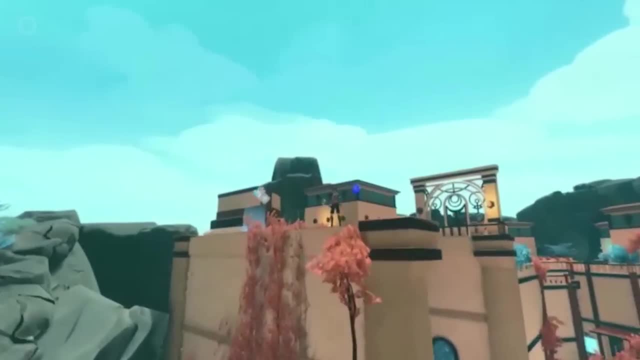 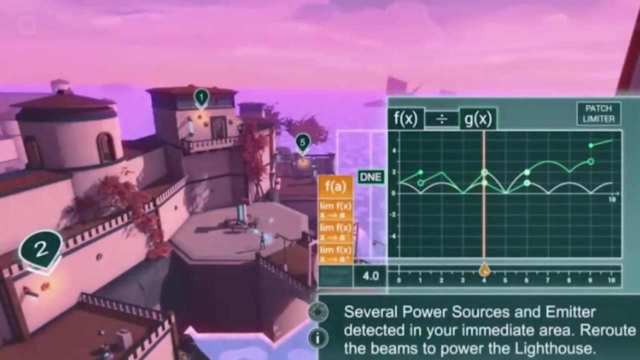 And use their experiences within the game to construct and retain calculus knowledge. Variant Limits promotes conceptual understanding through direct interaction and immediate feedback in the game environment. By providing students an opportunity to take a more active role in the learning process, Variant engages and motivates students like no other learning tool. 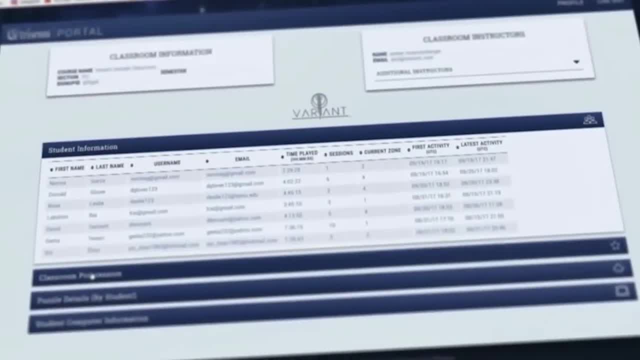 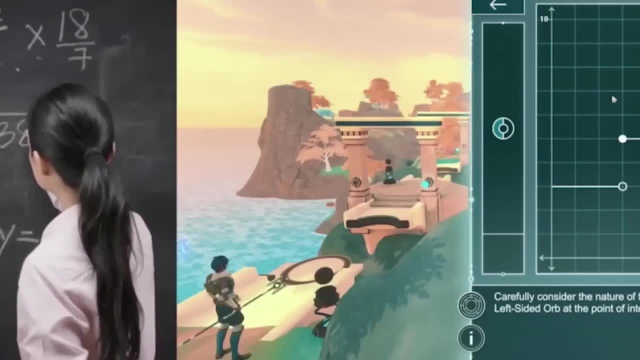 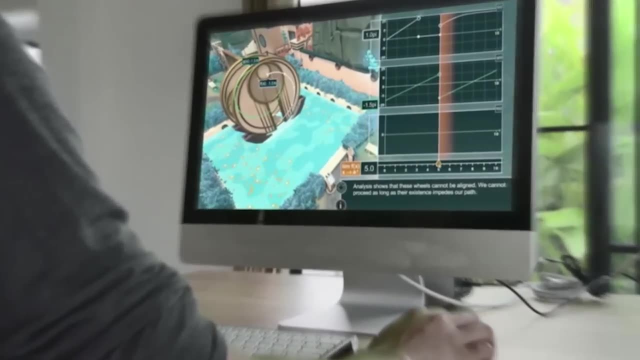 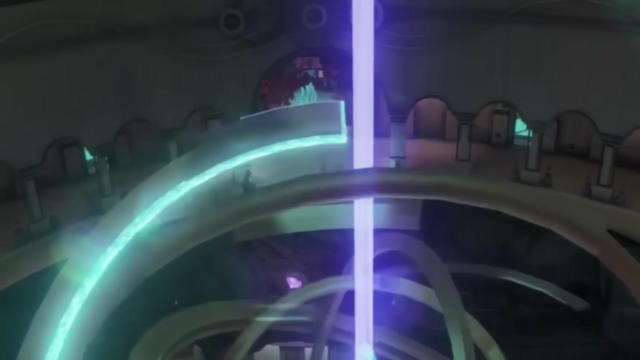 As students. advance learning is recorded via the instructor portal, which provides detailed information and tracking tools. A revolutionary new way to teach calculus, An innovative tool to empower and engage students. The first in a series that will transform the calculus experience: Play to learn with Variant Limits. 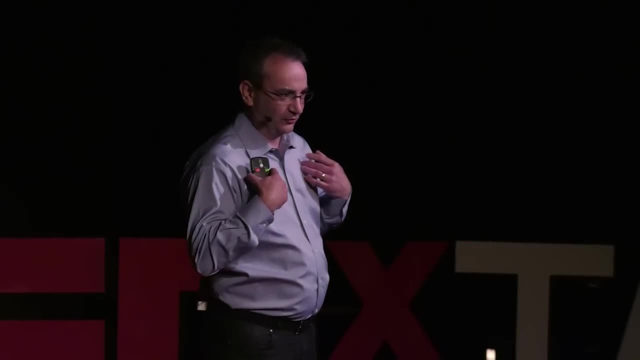 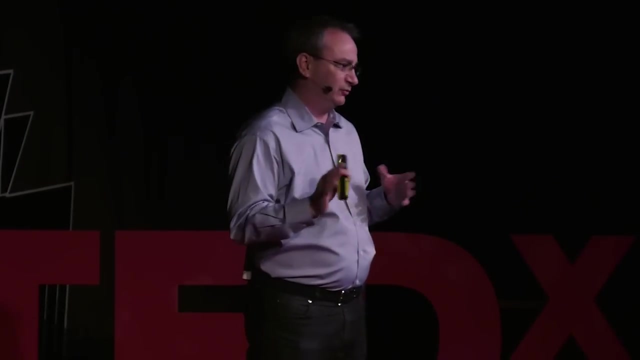 Now I can tell you this looks like homework I want to do. but the data speaks for itself. Students' homework play an average of ten times between two and four hours. I don't know any other homework students are willing to do. They're willing to do that often to get better. 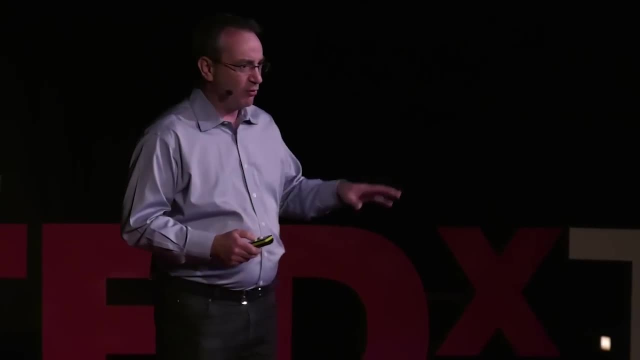 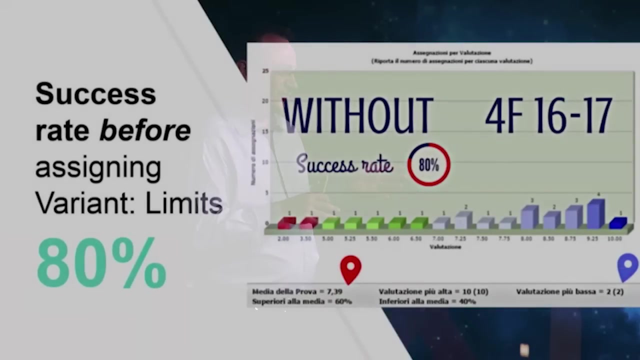 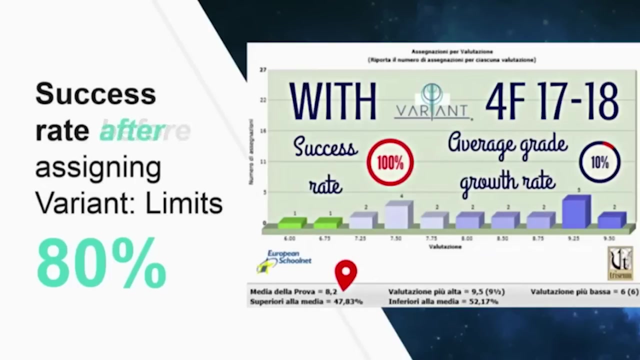 To master a subject, And while our own studies are still ongoing, a teacher in Italy recently used this game in her class. Last year, 80% of her class succeeded. It was pretty good. This year, the first time she used the game in her class, 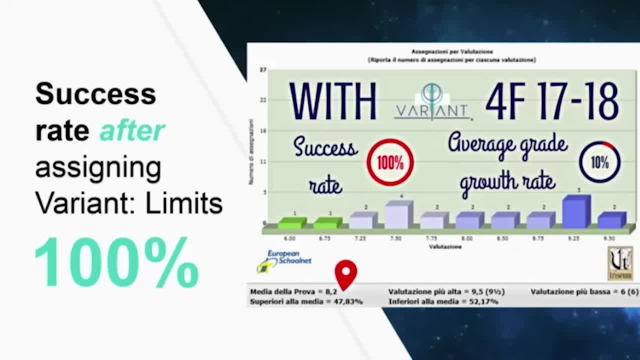 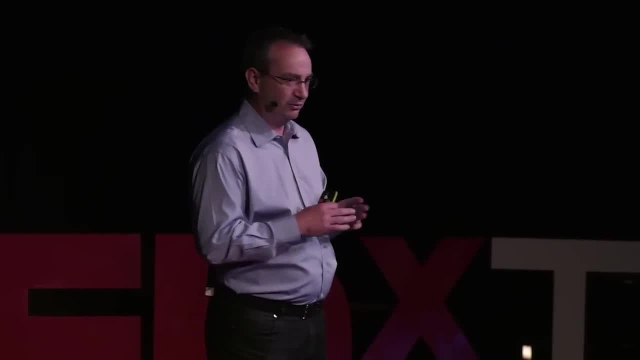 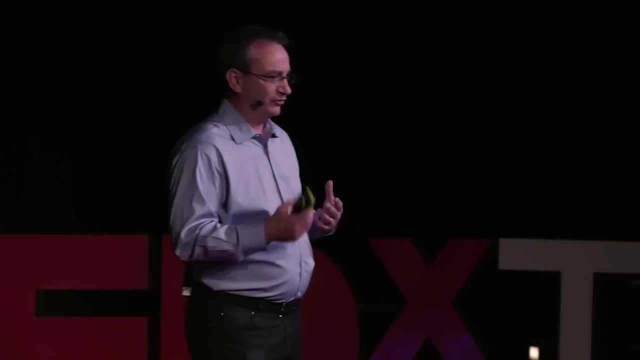 and the rate went to 100%. Everybody mastered the subject. Not only did they master the subject, but the average grade went up By about 10% across the entire class. Now, that's pretty powerful And the feedback we're getting from students and from teachers. 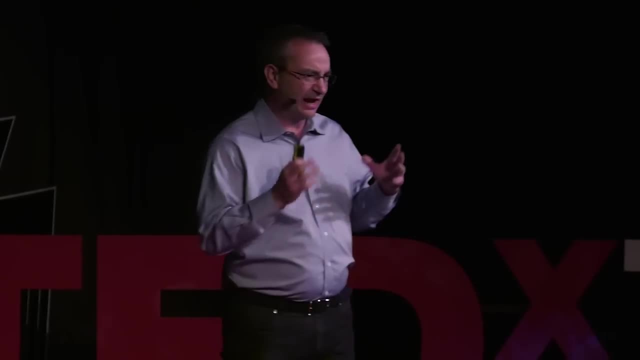 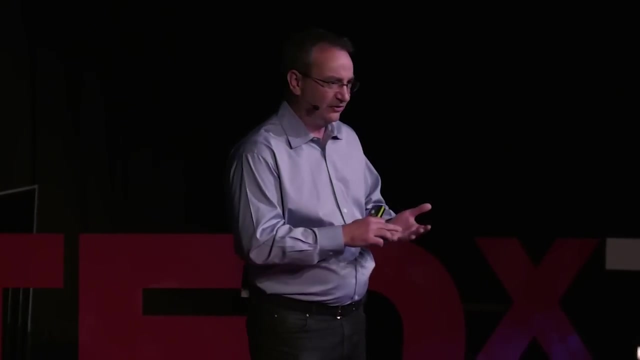 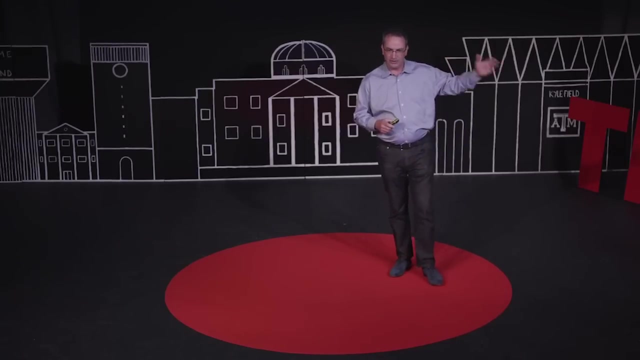 the engagement is overwhelming. See why did we create it? Because you heard, many students are failing calculus, And calculus is a foundation for any science, technology, engineering, architecture, business. Everybody has to do calculus. We have students enrolling in West Texas College, for example. 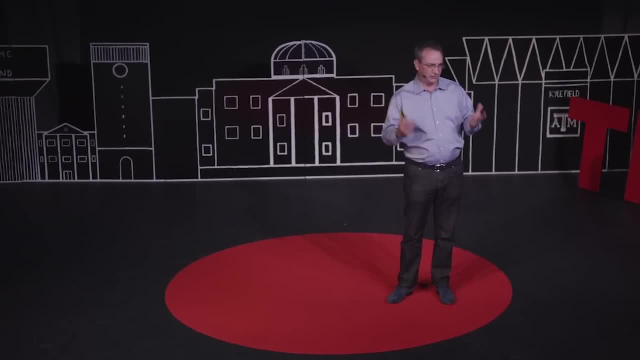 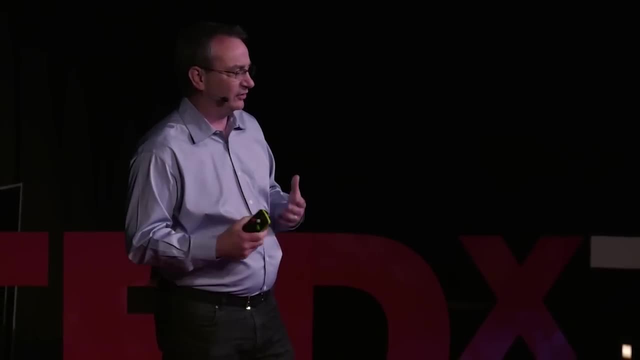 to get their calculus credit, But they don't really learn calculus. What are we doing? We're not helping them. Is there another way, another tool that we can give teachers and students to really help them? Recently, a young lady came up to me at a conference and asked: 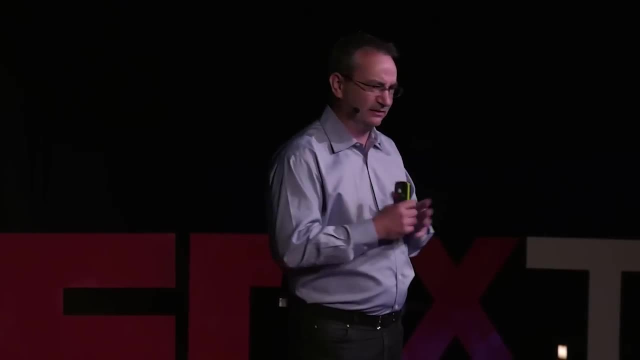 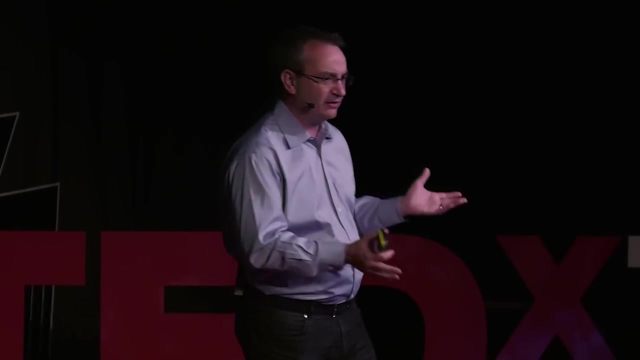 so do you like math? Oh my God, I hate it. Whoa, Very strong words. Yeah, I'm in the classroom and the teacher keeps on going and I can't keep up. So I'm paying $300 a month on tutoring just to keep up. 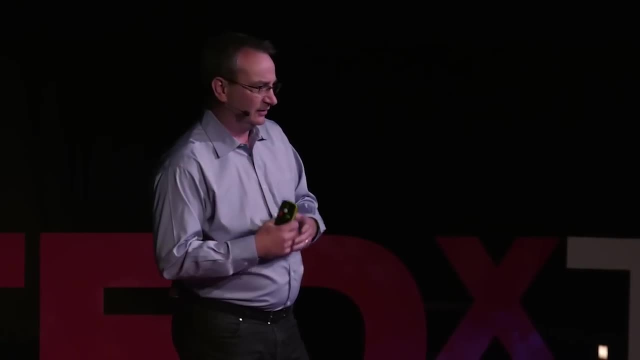 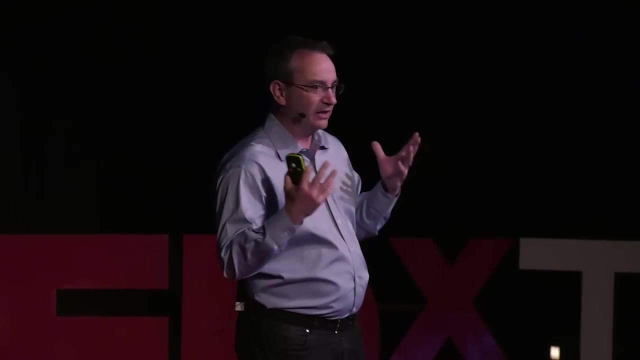 because I know I'm going to need it in college to succeed. But do you like games? Yeah, I play games. Well, sit down. She sat down and within an hour she's like: oh my God, I actually understand what this is about. 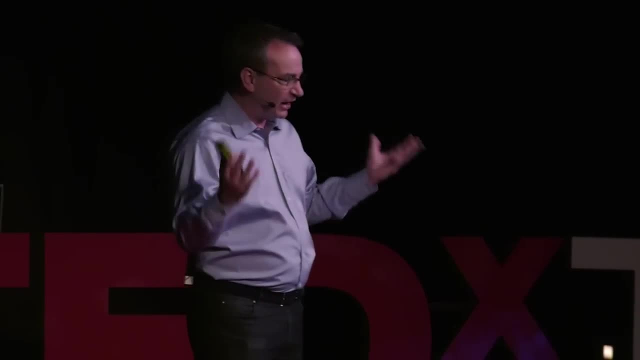 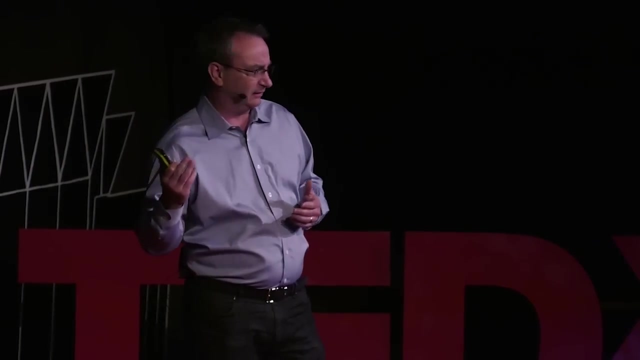 And math is so much fun. I didn't realize it could be so much fun. Why shouldn't learning be fun? That's how we start off. Think about failing in classroom. What do you get when you fail? You get an F. 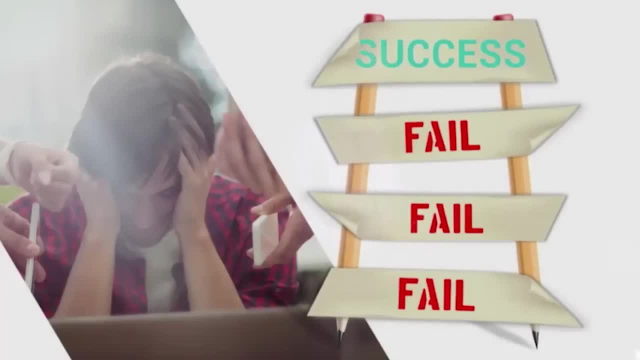 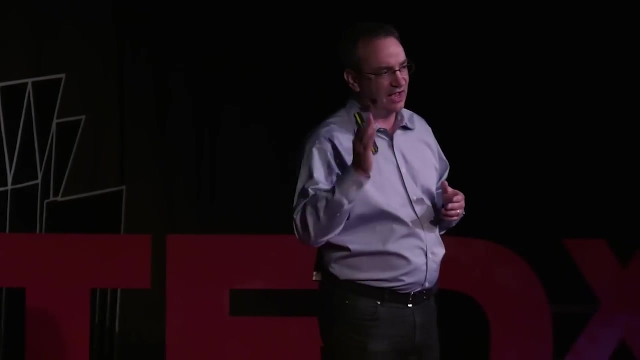 OK, well, let me try that test again. And another F. How motivating is that? Not very much right? Nobody likes to fail. That's how we grade. In a game. you can't succeed, You can't finish a game unless you master it 100%. 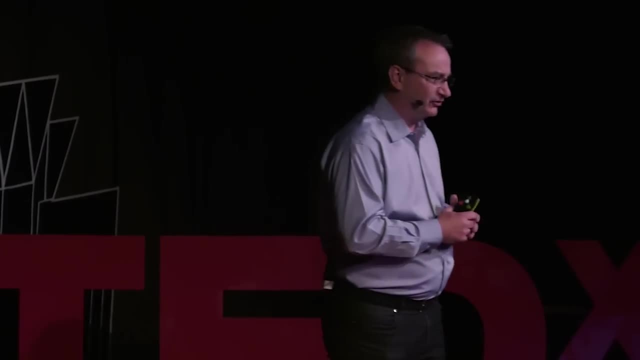 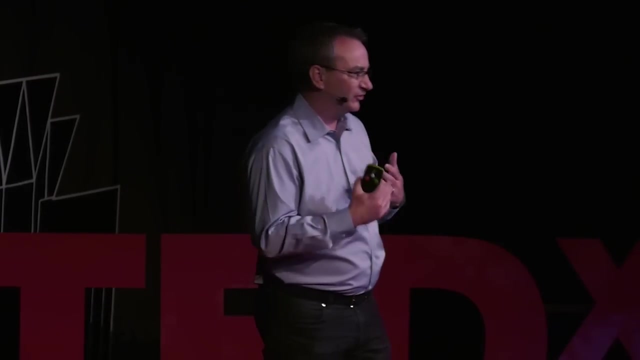 You can't get to the next level with 98%, You have to get 100%. And not only do you have to get 100%, failing is fun. That's why students play over and over again and you say, oh my God, I actually understand what this is about. 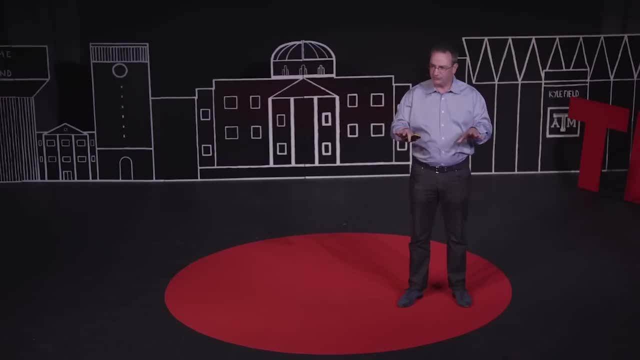 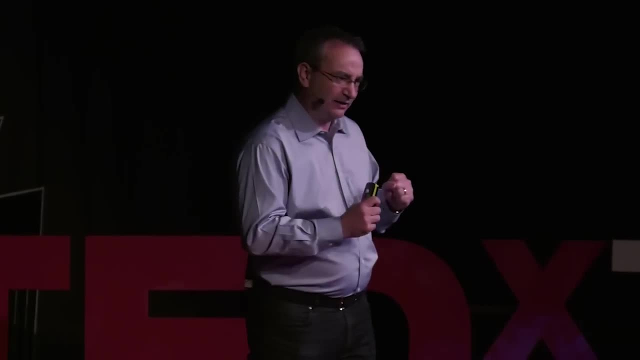 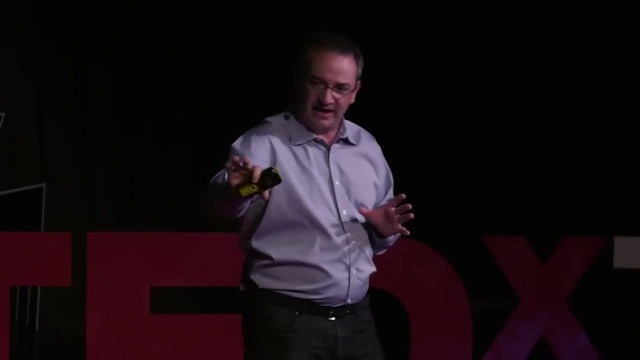 And you see that with many games Highly motivational. Imagine the situation. You're about to get to the airport. Thankfully, the pilot is fully trained. Airplane is fully working. You run. You're kind of running late As you reach the gate. the airplane is just pulling off. 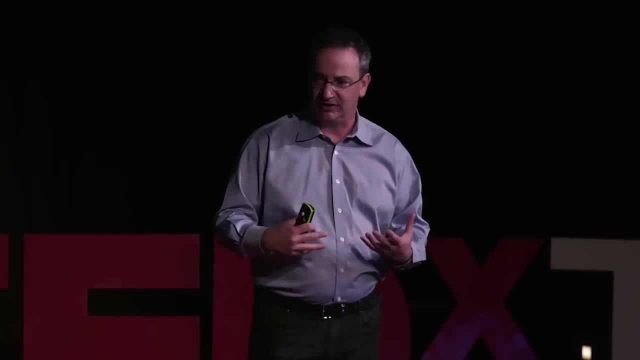 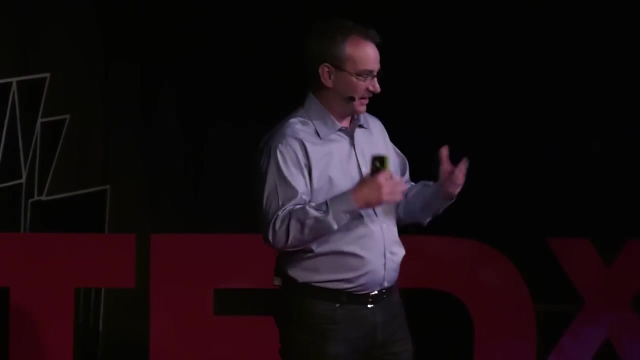 There it is, The window seat that would have been yours. it's empty. You're standing on the other side Right now. First, you're going to be upset. Obviously, I'm not going to repeat the words that I've heard. 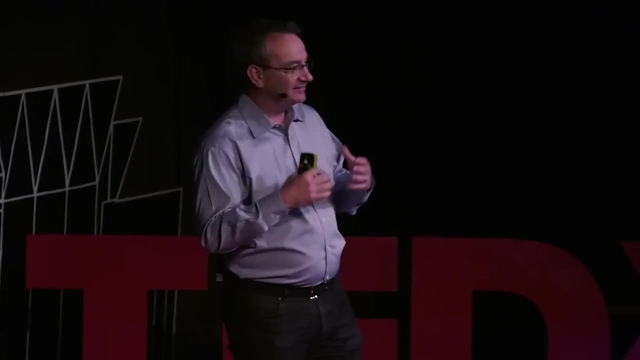 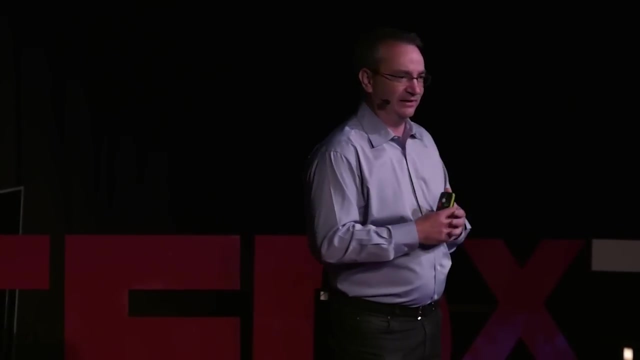 that people say in that situation, And when I've asked what's the next thing that goes through your head, Most people say: well, we're going to start planning. How do I get to my destination? Well, that's actually the third thing. 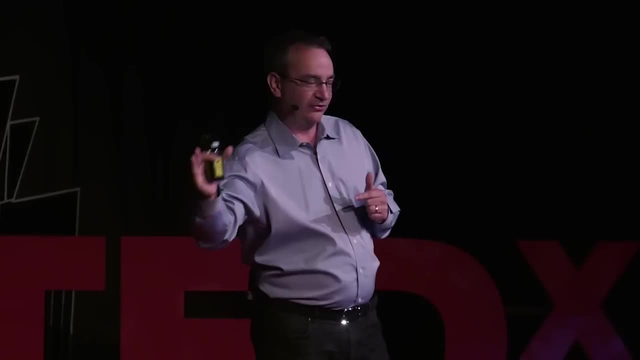 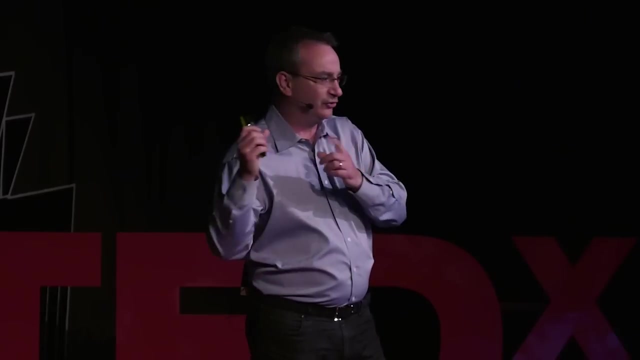 Number two: you're going to think back on all the things that if they would have just done a bit better that would have made you sit in that airplane. The security line if it would have just been a little bit shorter. The bus if you would have just been on time. 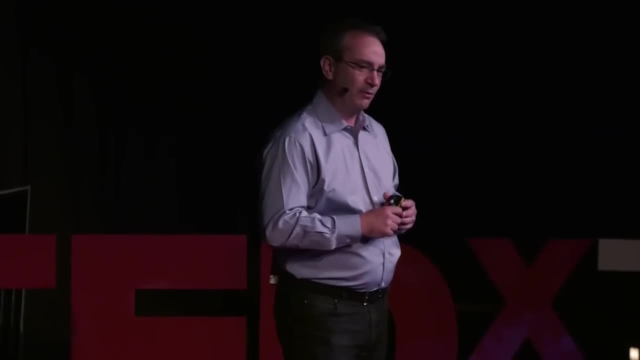 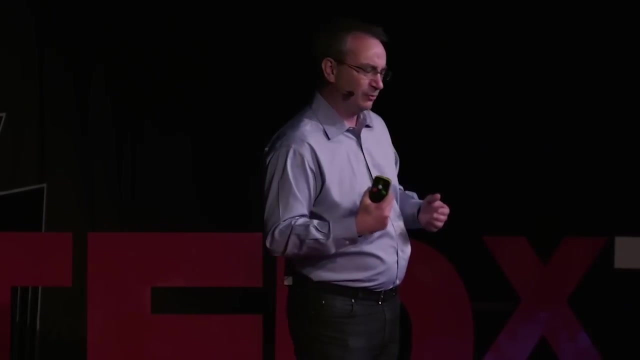 I could have made that plane. Well, what if I can tell you I can rewind time and give you another try? You want to have another go at it? Do you want to try to get that airplane to go home for Christmas to see your family? 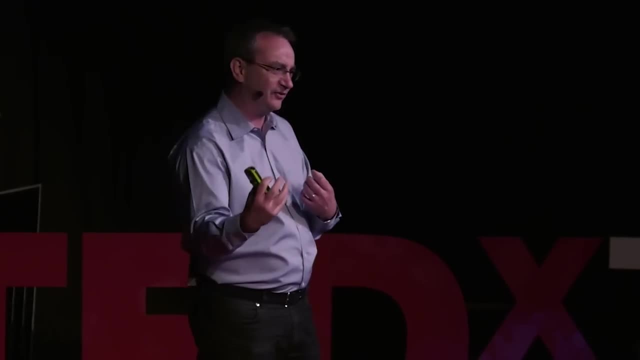 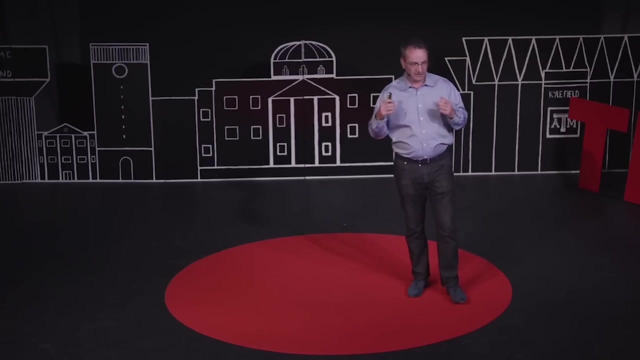 Who's going to say no, You can't see it, It's right there And you know what it's going to take to succeed. Yes, of course I'm going to try. Well, unfortunately, in real life that doesn't happen. 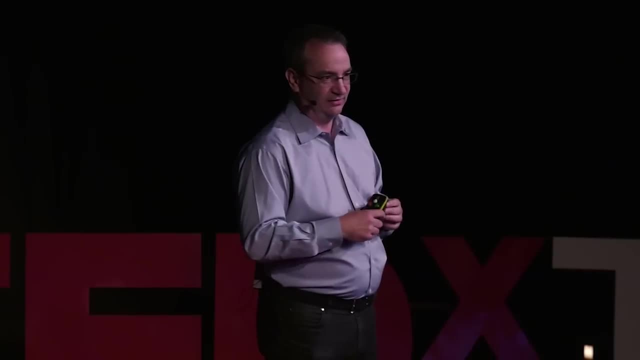 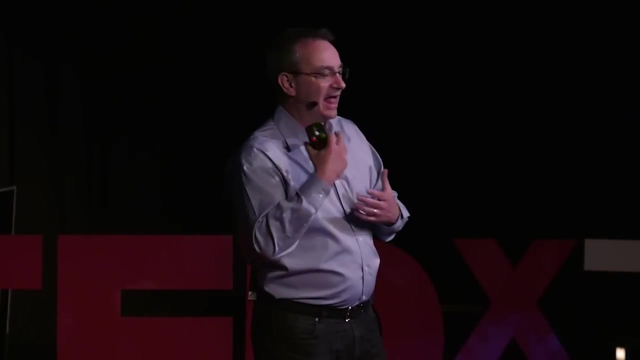 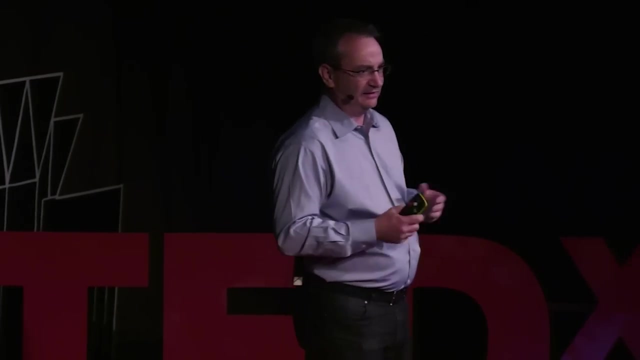 But in a game I can rewind And you can try again And I can show you what success looks like and how you get there. And that's the power of game-based learning. We've taken this to a whole new level right here at Texas A&M.